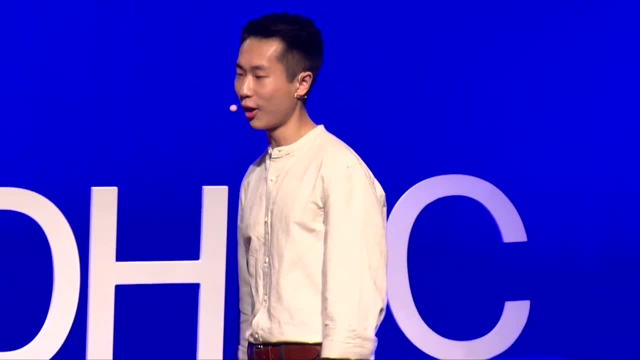 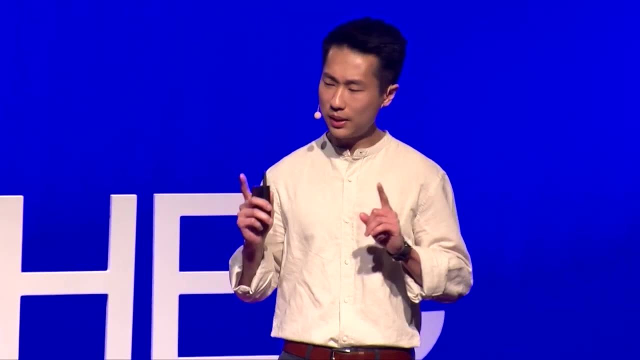 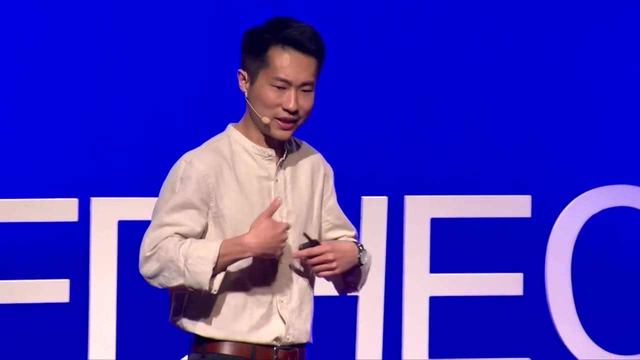 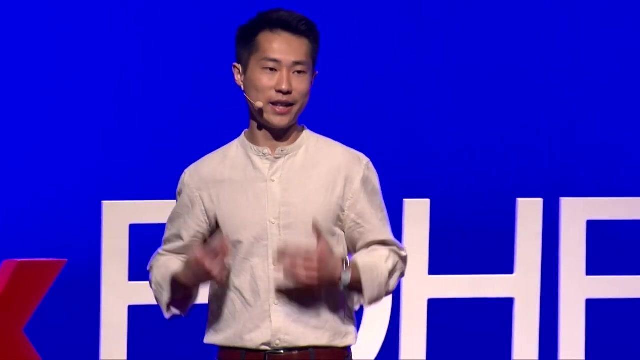 and, more precisely, how I overcome the toxic comparison in my life. To start with, maybe you're wondering: wait, maybe this guy never faced any comparison in his life, right? But that's wrong. Let me tell you why. Maybe it's obvious enough. I am from Asia, and more specifically, a place called Hong. 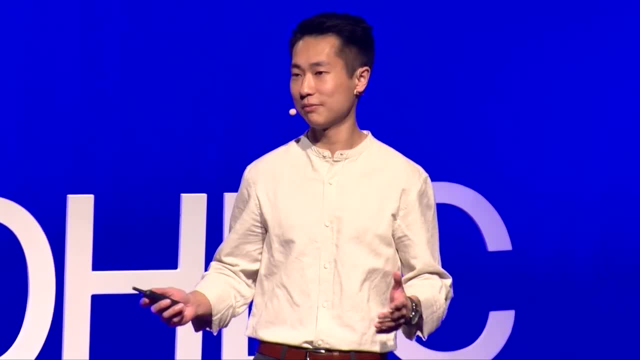 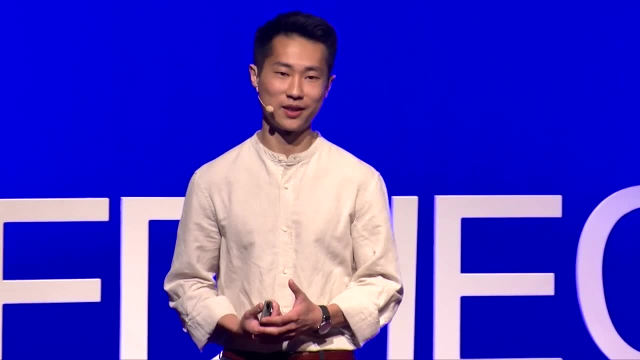 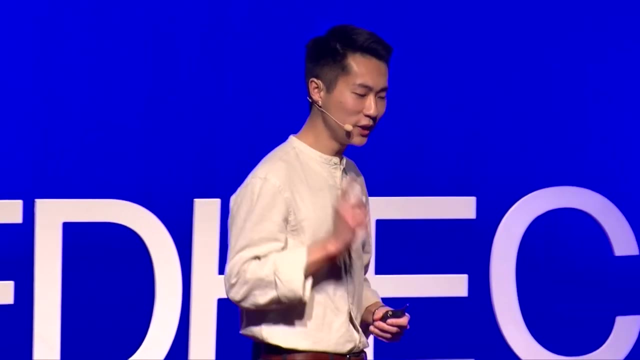 Kong. And if you have no idea about Hong Kong, that's okay. I give you one fact about Hong Kong. We Hong Kongers like to compare. Comparison is deeply rooted in our culture. When we were young, we fight hard to get into a good school. We fight hard again in public examination. 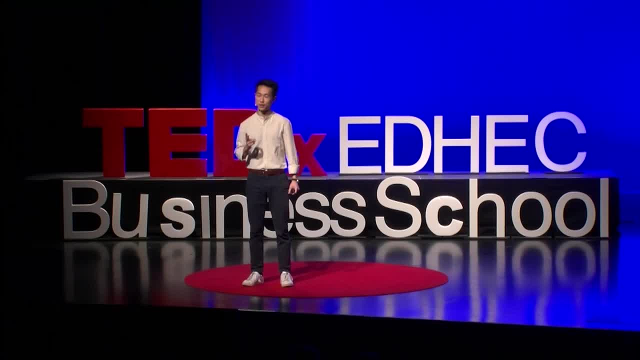 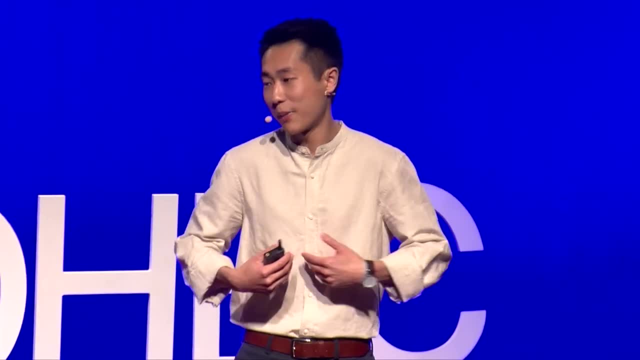 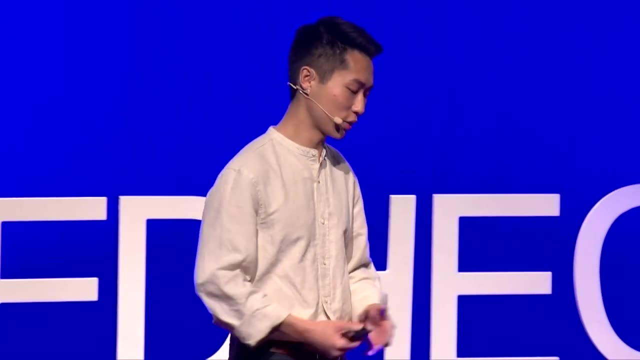 because that examination selects only around 20% of us to go to university And then an internship, a job. we compare ourselves with other people on where we live, whether or not we have an attractive partner, et cetera, et cetera. 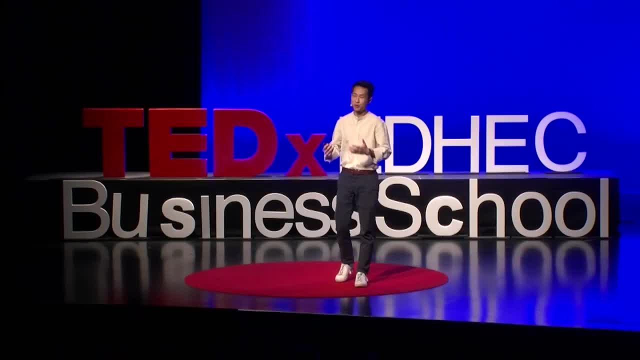 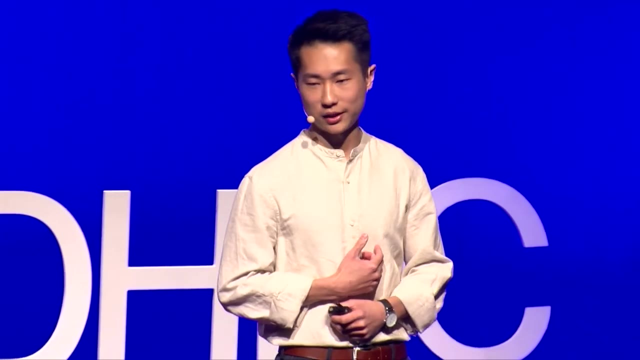 Comparison is something that I grew up with, and perhaps just like most of you, And one of the most recent examples of me handling comparison is actually coming to this beautiful country, France. In 2019, I finished my bachelor in Hong Kong and, instead of finding a job immediately in Hong Kong, 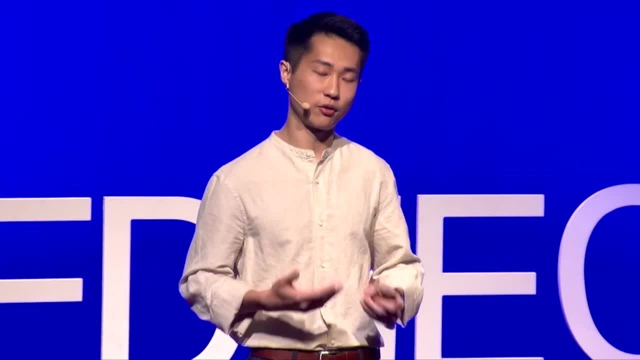 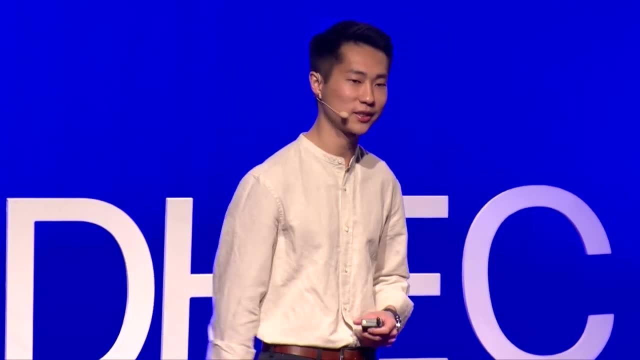 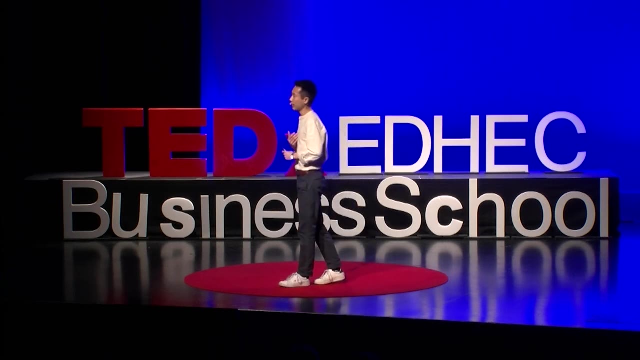 I decided that I want to do a master's degree in France. However, it was a very rare decision because in Hong Kong people mindset: we like to maximize our gains in the shortest period of time, Especially in my case. I studied in a fairly good university in Hong Kong. 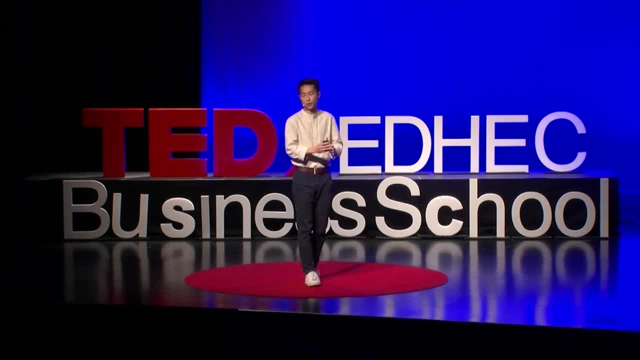 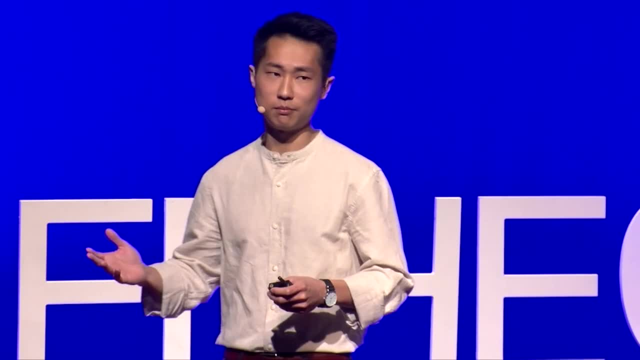 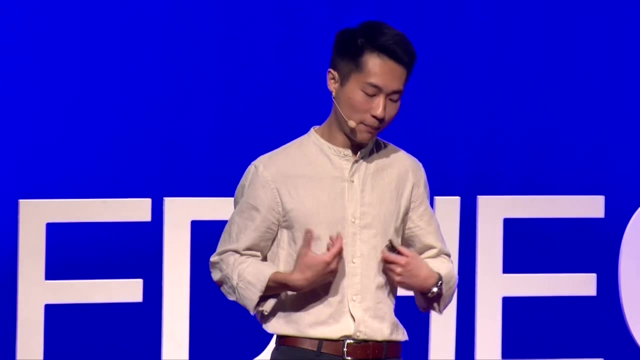 So finding a job for me is the most straightforward and safest option for me. Well, indeed, when I see my friends- many of them- they find a very good job and they have a very good foreseeable career path ahead of them. Well, comparatively, 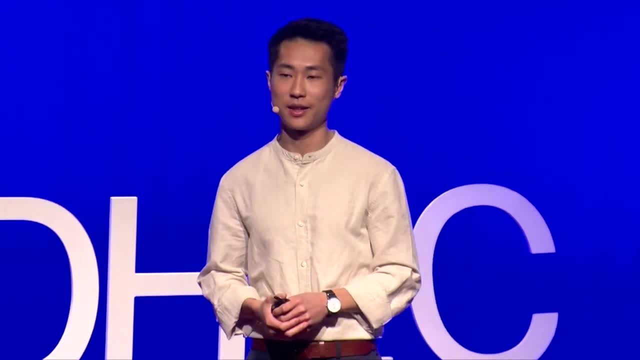 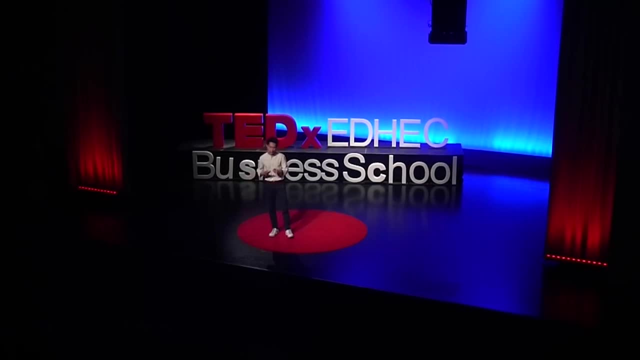 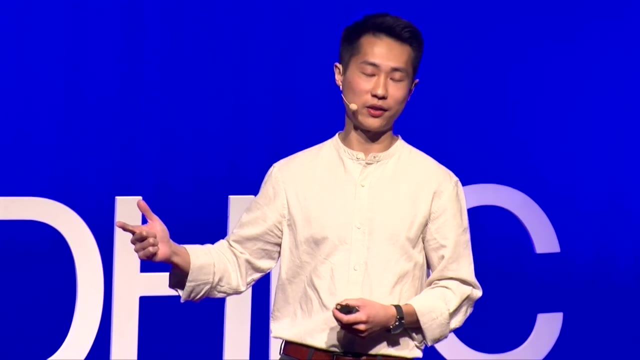 I am going to complete opposite of this mindset. Now I am spending three extra years in a complete new culture, trying to construct something in my life. When I first came to France, I didn't speak the language, I didn't have any network. 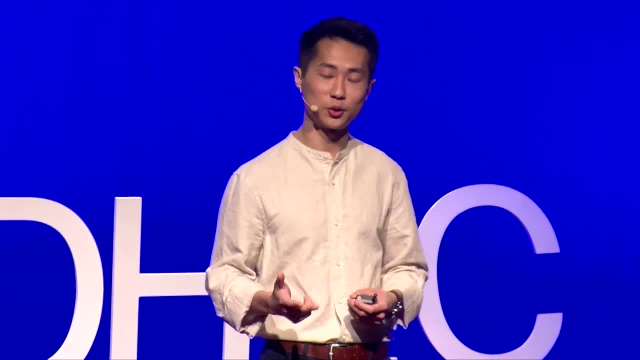 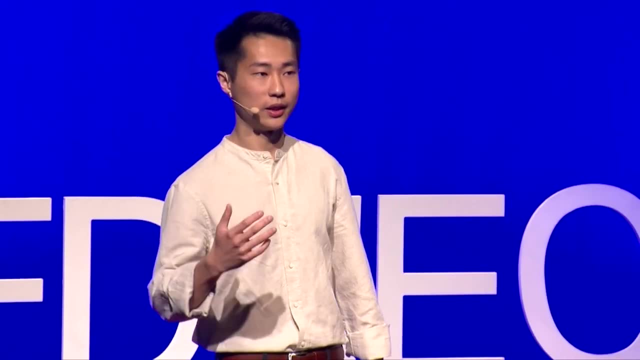 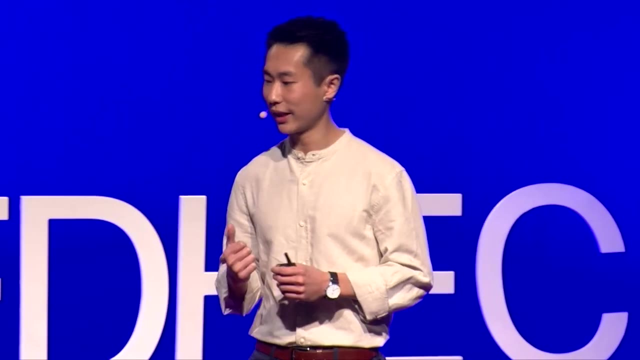 and all I have is so many unknowns that I have to deal with, And perhaps some of you can relate to this story. In our life, life is usually decent, right Until the comparison kicks in. When comparison kicks in, we feel insecure. 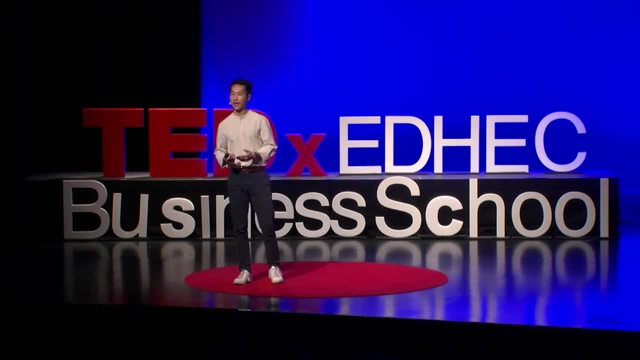 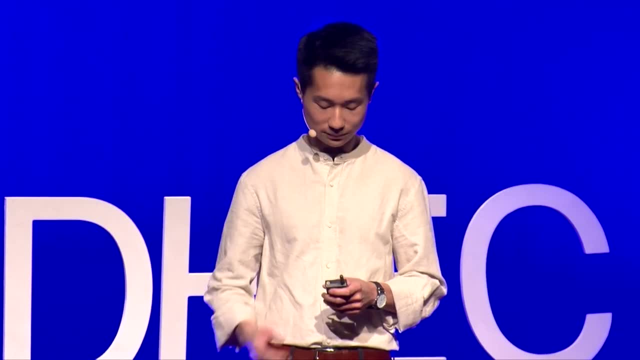 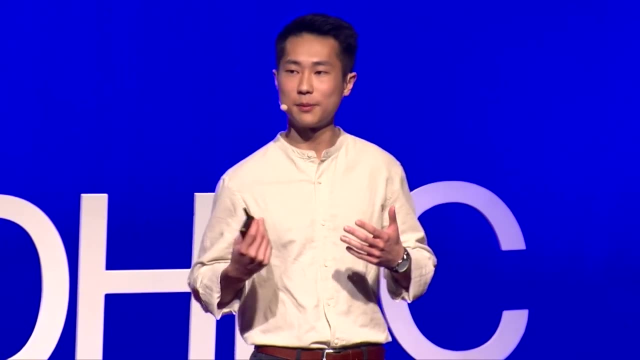 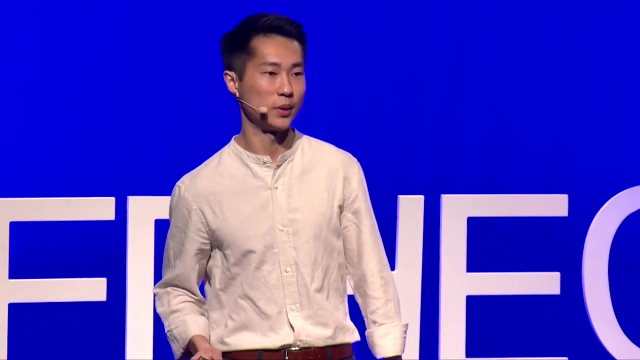 And today I want to share to you how I see comparison differently now, and I hope that my ways can help you also. First, it's about time. When I compare myself to other people, I always look at the time frame instead of a particular time moment. 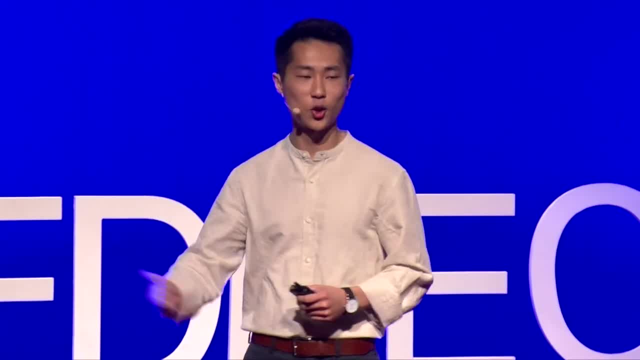 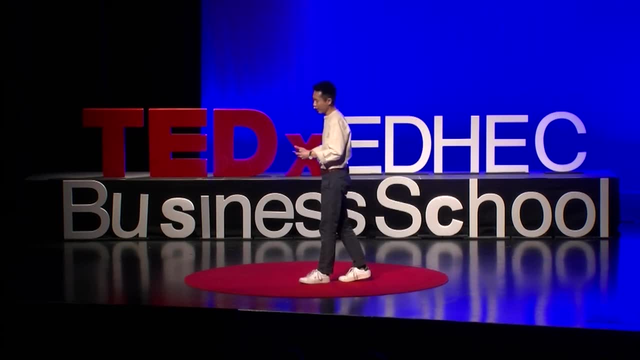 In today's fast culture, we want everything to be so fast. We order something online, we want them to be delivered in one second. We post something online, we want the reactions, we want the likes right away. Indeed, we should be grateful. 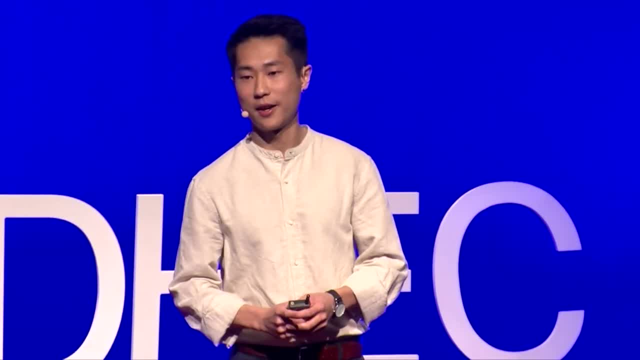 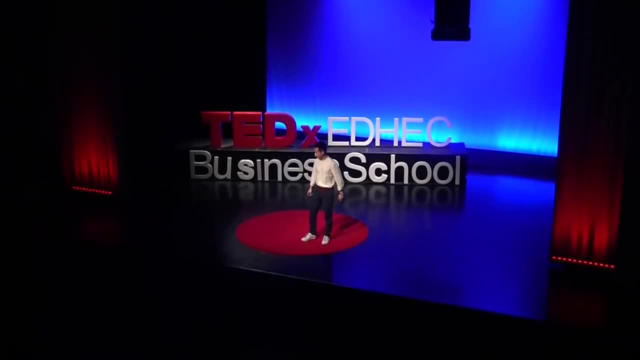 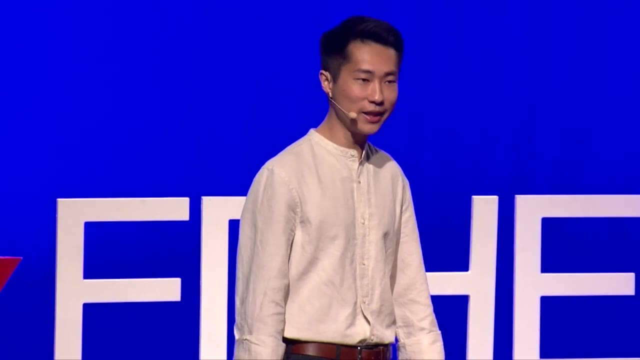 that technology has speed up a lot of things, but if we want everything to be so fast, it is extremely dangerous in comparison, And to understand this, let's think about who we compare to most of the time. Today, I am fortunate enough. 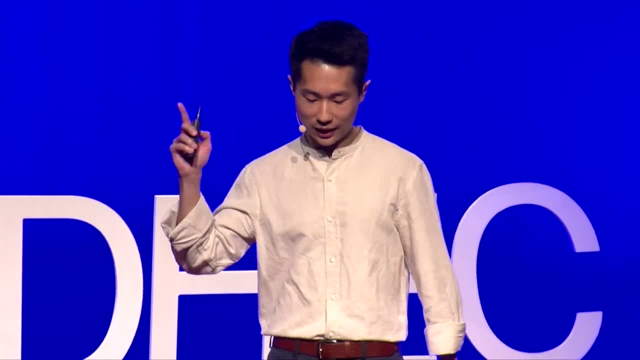 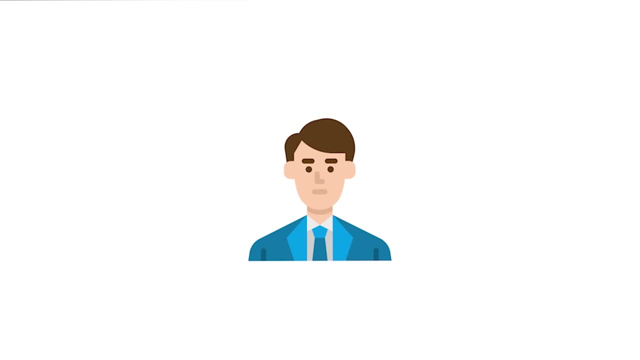 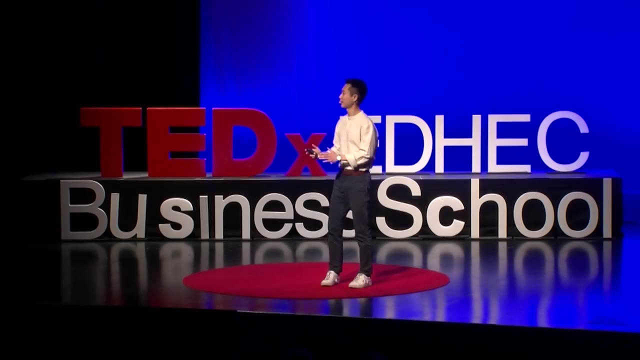 to bring two friends with me. First, let me present you Michael. Michael. he is a young, good-looking, smart investment banker who likes to post on LinkedIn to share how good he is. Of course, he is rich, stylish, intelligent. 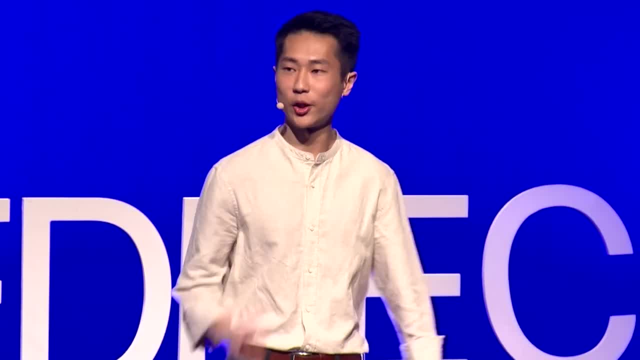 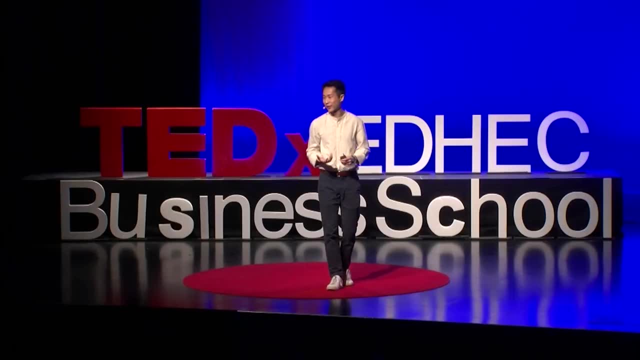 and we often compare ourselves to him right. First, because you always see him on LinkedIn, But also we all like to achieve amazing things and reach the top spot, that everyone can recognize us. Then let me introduce Mary. Mary, she is a beautiful influencer. 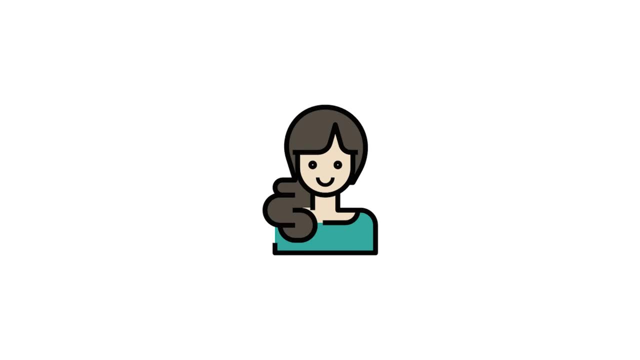 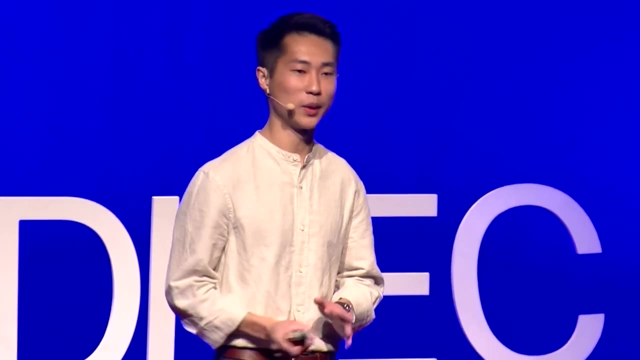 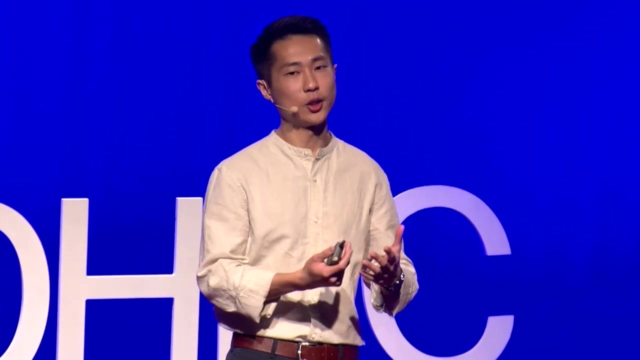 on Instagram with more than 200,000 followers. Her favorite activity is to share her favorite hotel and also restaurant, no matter where she goes. Again, we like to compare with Mary, because who would say no to that influence and lifestyle that she enjoys? 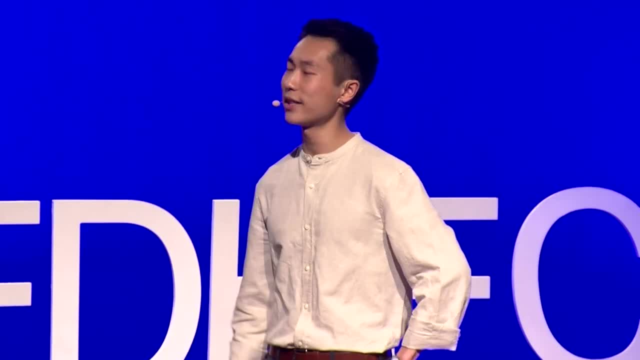 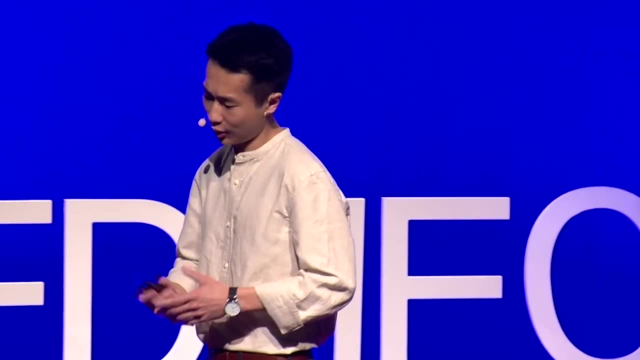 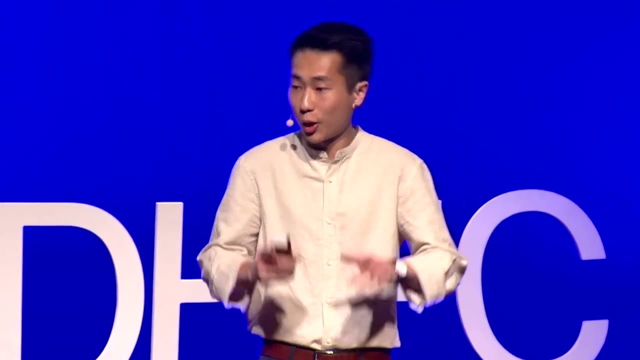 However, maybe there is one thing we seldom pay attention to, and that is they are actually very rare. Well, in fact, you won't really see lots of them in the street And, more precisely, they are the top 1%, if not the top 0.1%, of the people in that domain. 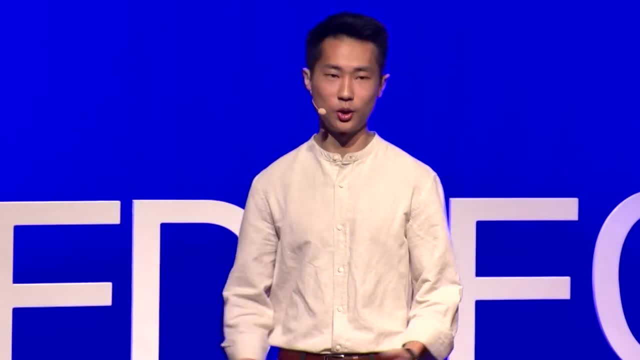 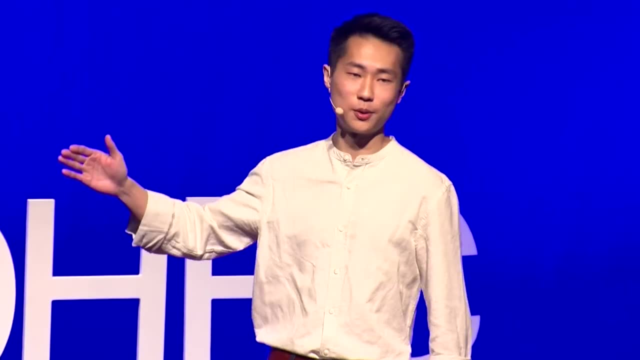 And today I don't want to say anything like you know what, Just compare yourself to the average people, Because I know that if you compare yourself with other people, you compare yourself to the top people, And to me that's normal. 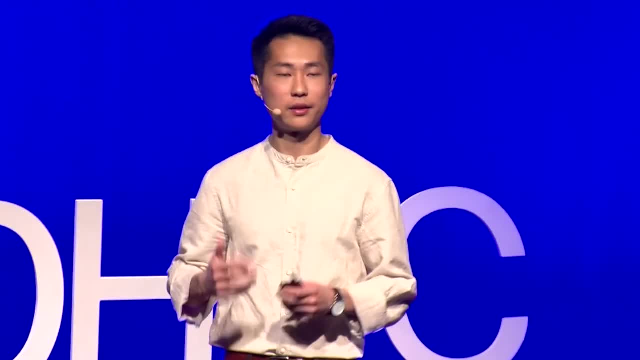 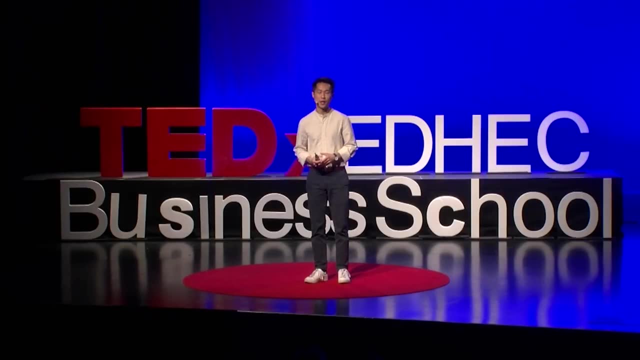 But the question is: do you give yourself enough time? In today's fast culture, we want everything to be so fast, but achieve amazing things requires a lot of time. When we do comparison, we very often look at the time, at this particular moment. 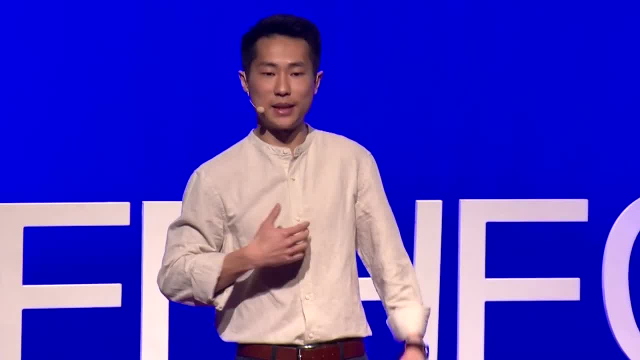 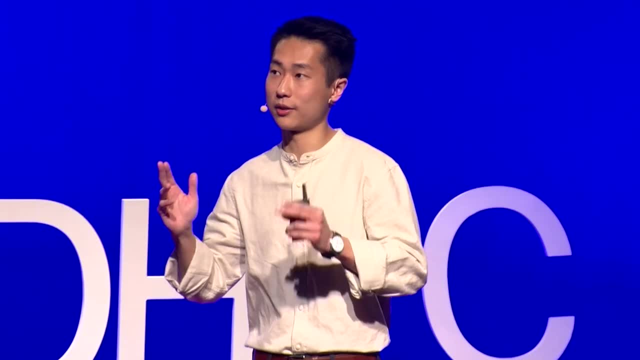 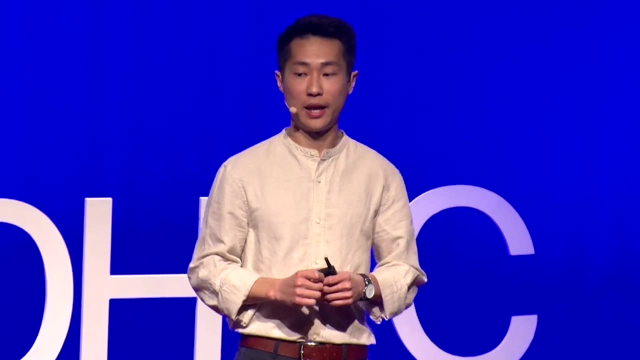 For example, my friend has a better achievement than me now, so I am sad, But then, unfortunately, we seldom really look at the future and we seldom give ourselves enough time to achieve amazing things. And that's the first lesson I learned in comparison. 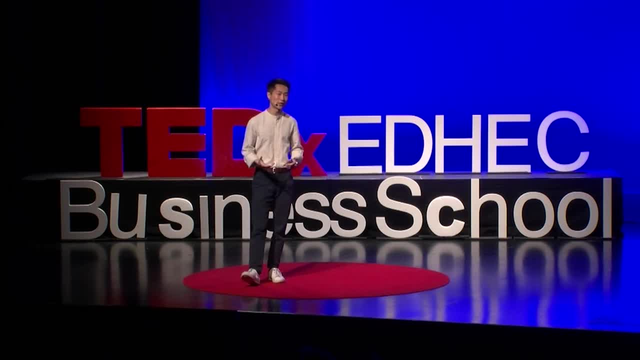 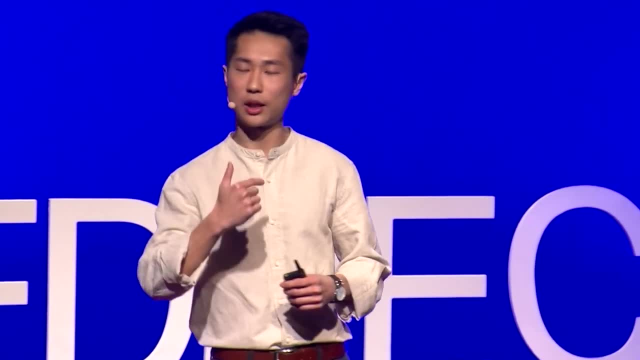 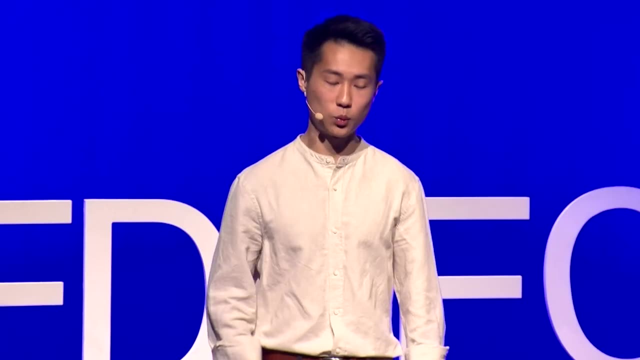 We basically spend a lot of time to think how we are worse than other people, but we are not so lenient to ourselves. We seldom give that time to ourselves to achieve great things. The second reason why we suffer a lot from comparison is also because 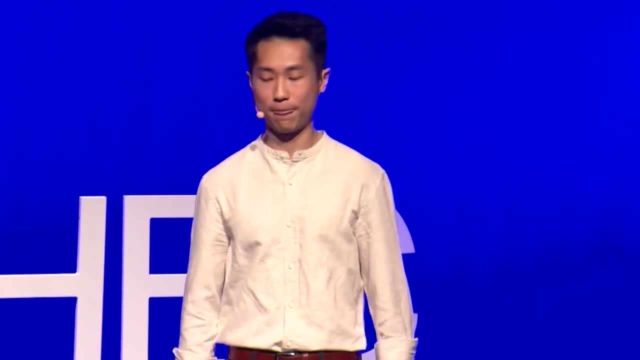 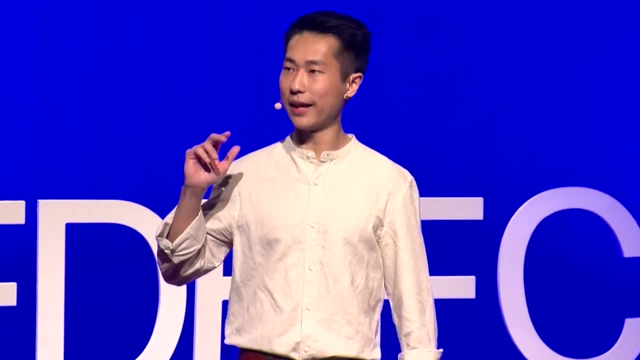 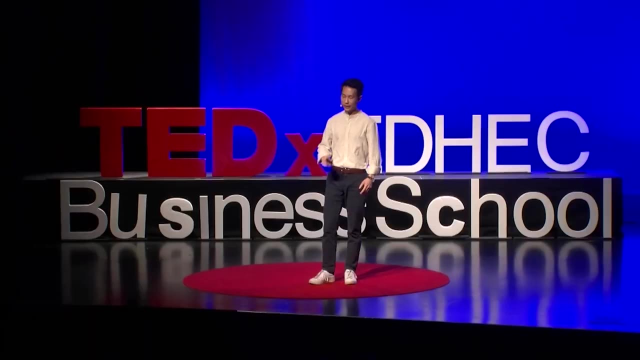 the way how we compare to other people. When we compare to other people, very often we like to compare to different people at their perfect side. I know that sounds very abstract. Let me give you an example again. Imagine Michael. again, Investment banker likes to compare, also right. 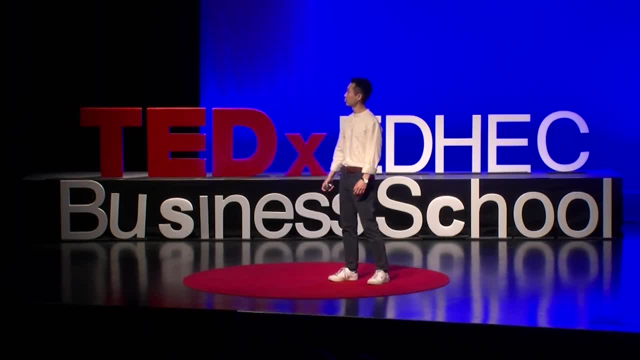 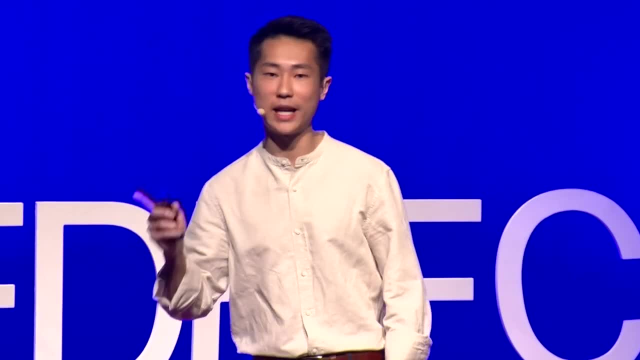 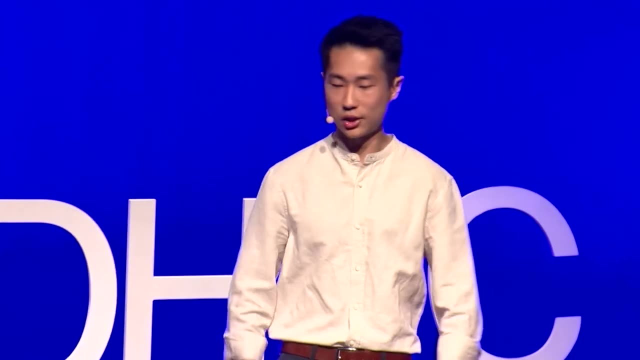 And Michael. if Michael wants to compare to Elon Musk, you know what Michael would not do. Michael would not compare every aspect of his life to Elon Musk, So he would not compare, let's say, intelligence, family study, etc. etc. 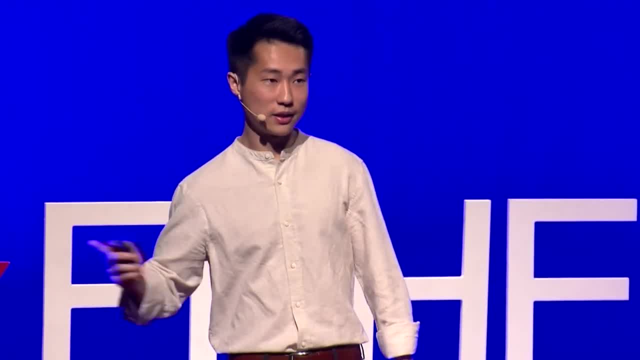 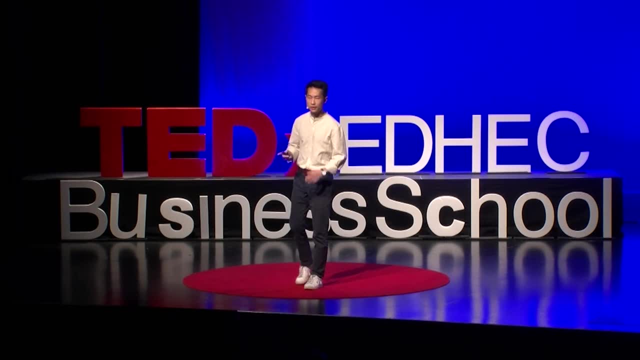 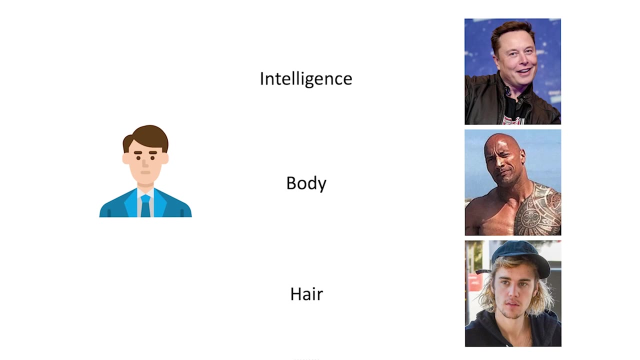 to Elon Musk. Instead, what Michael would do is the following: Michael compares his intelligence to a very smart person like Elon Musk, then his body to a very strong person like Dwayne Johnson, then his hair with a very beautiful person like Justin Bieber. 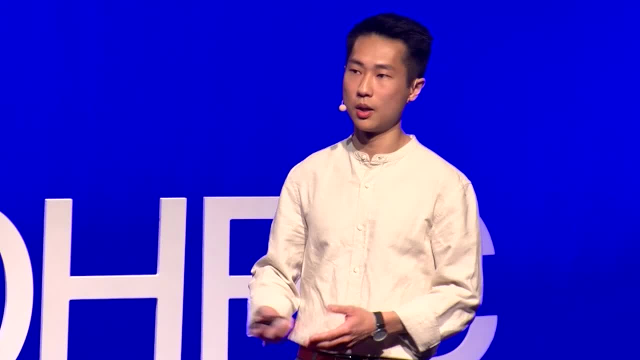 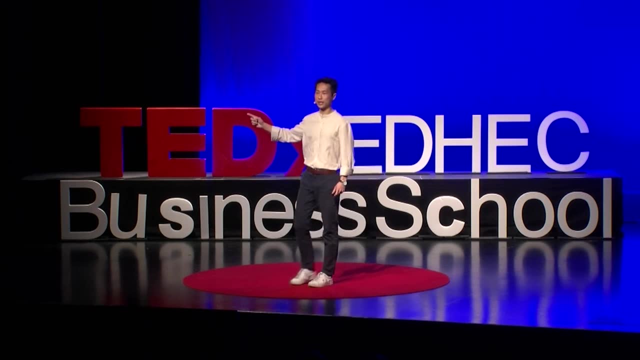 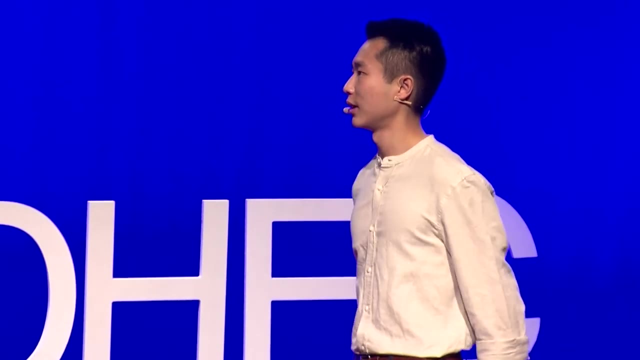 That's how we compare to other people. We compare to so many different people, and usually on one aspect, and that is their perfect side. Then let me show you one simple trick that you can turn the whole comparison around, But this time same people instead. 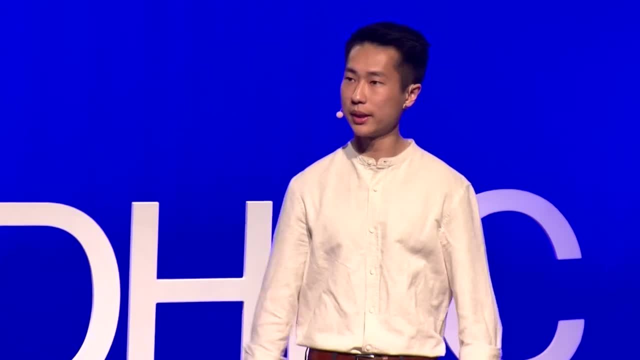 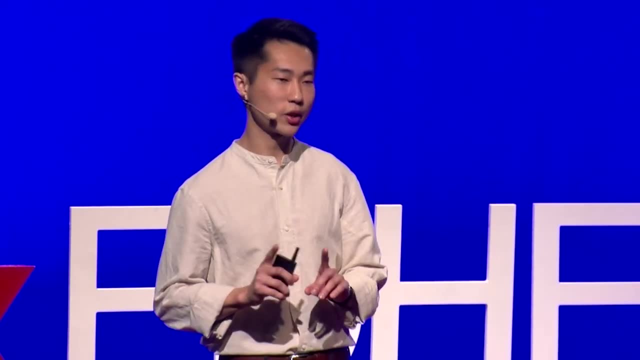 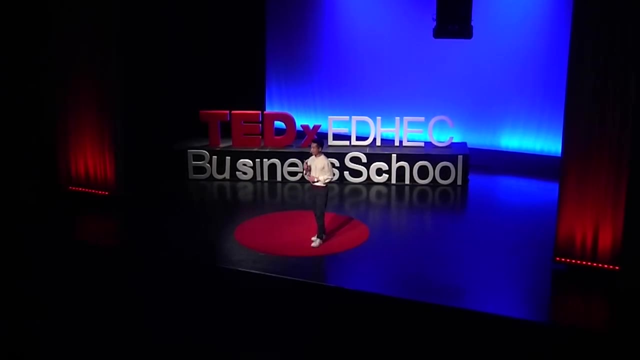 You compare your body to Elon Musk, your hair to Dwayne Johnson. But, by the way, hair is a very sensitive topic recently And if you can try not to compare your hair with other people And make sure don't tell a joke about hair. 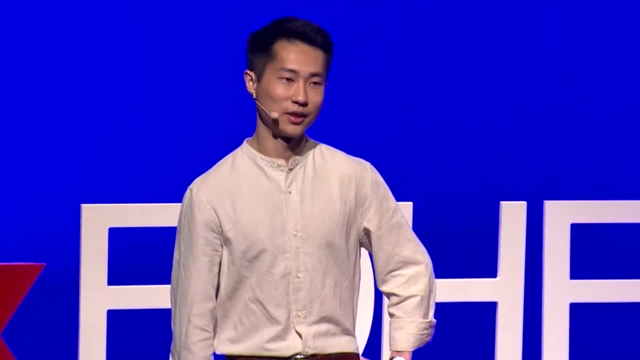 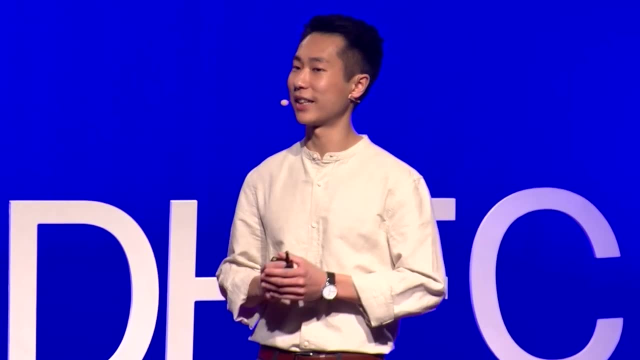 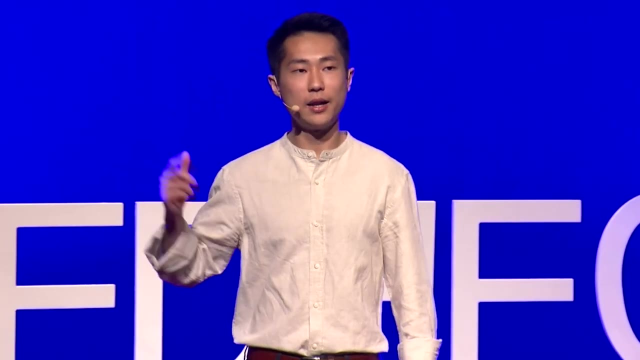 And what about intelligence to Justin Bieber? You see, by changing the angles of comparison, you change the whole comparison game, And that's what I do every time. When I compare myself to other people, I make sure that I put enough aspects and angles. 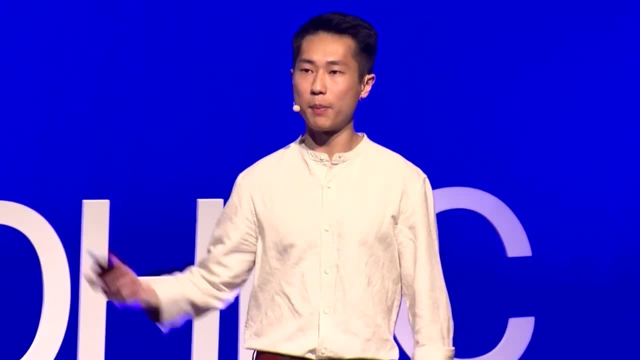 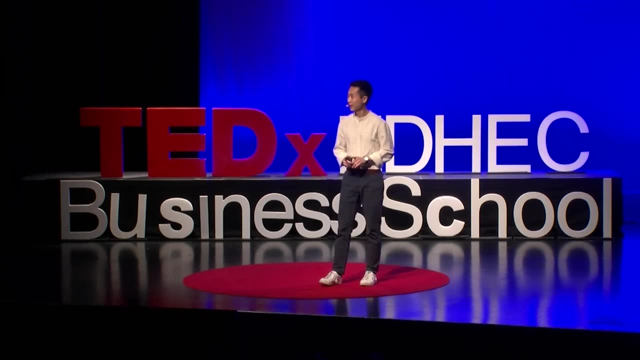 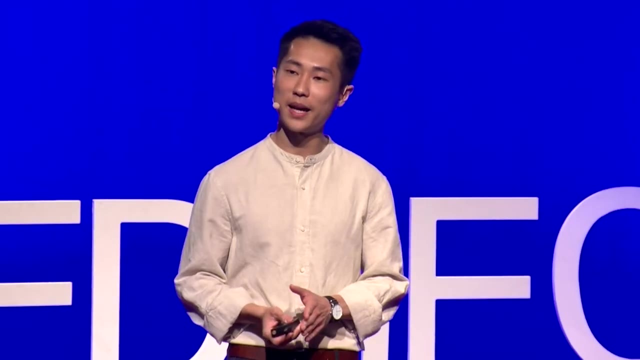 In my case. maybe that's true that people back home may have a better career than me, But I also have a better pain au chocolat. Well, I was just kidding on this one. But what about quality of life? I am now healthier. 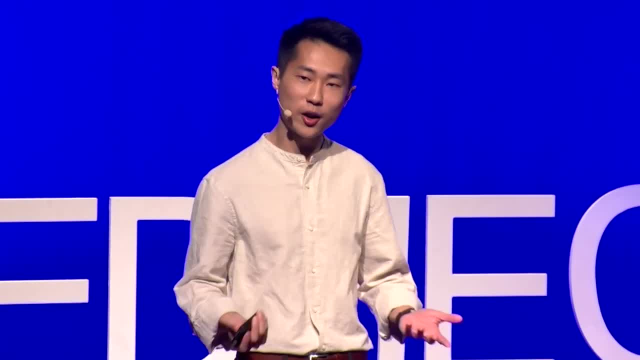 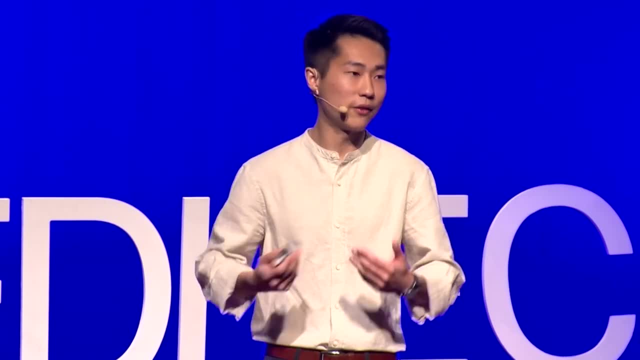 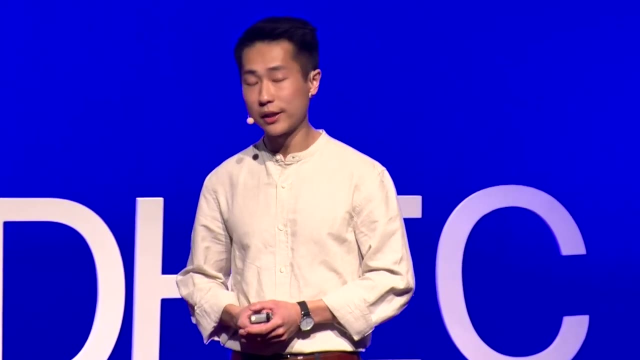 less stressed. What about new friends? Today, some of my friends came here to support this CCO And I've never met them if I've never came here. What about new culture? Before coming to France, I thought that French people are lazy. 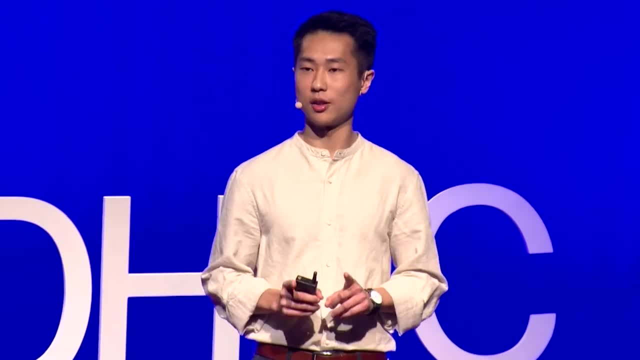 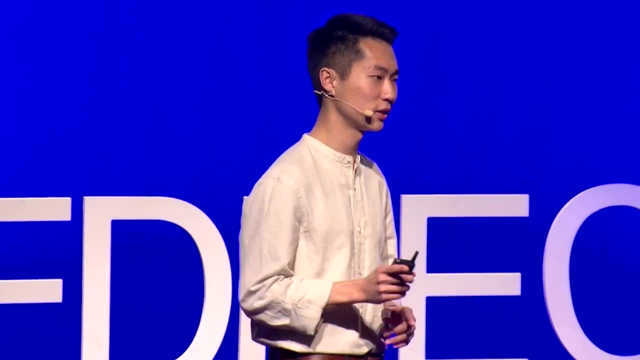 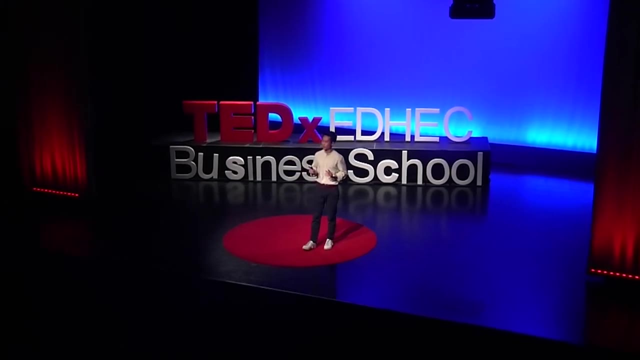 and they don't work. I was wrong. French people work a lot, But after they complain about work doing their apparel with friends. See, every time when I add new angles I change the whole comparison And of course your life will be so miserable. 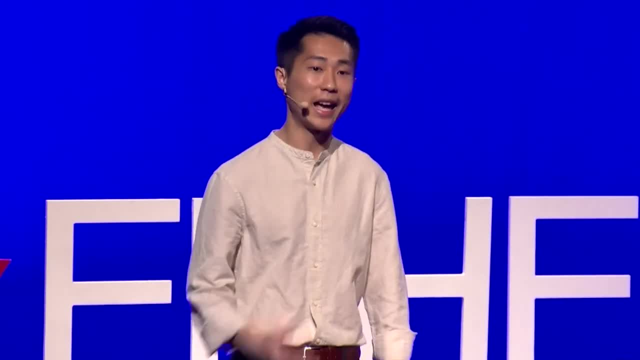 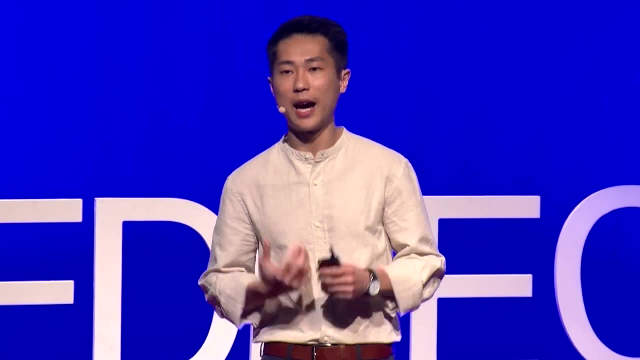 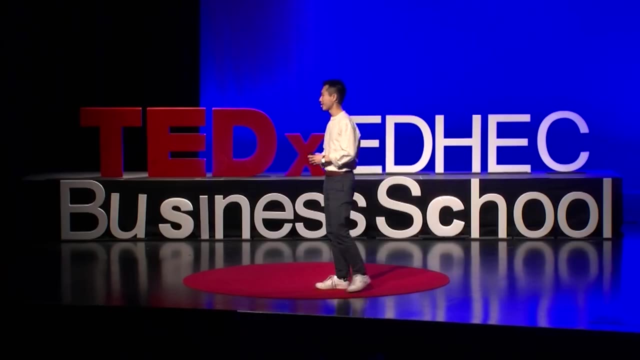 if you just compare yourself to different people at their perfect size. That's why, every time when I believe that my life is miserable, I try to see things from more angles And, honestly, every time when I do this, I realize that there's something I can be grateful for. 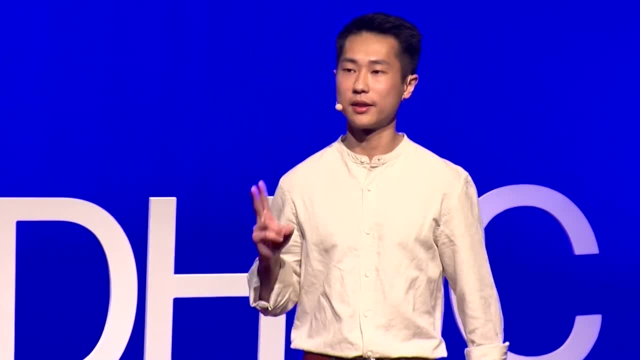 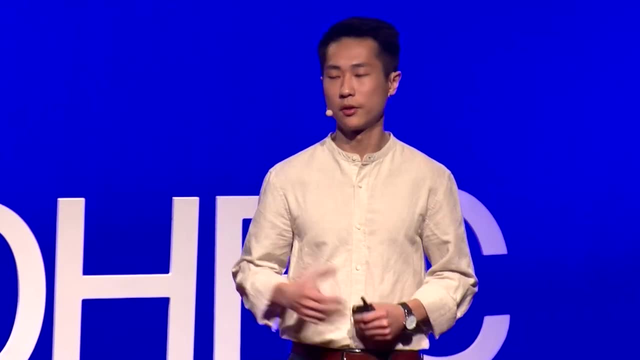 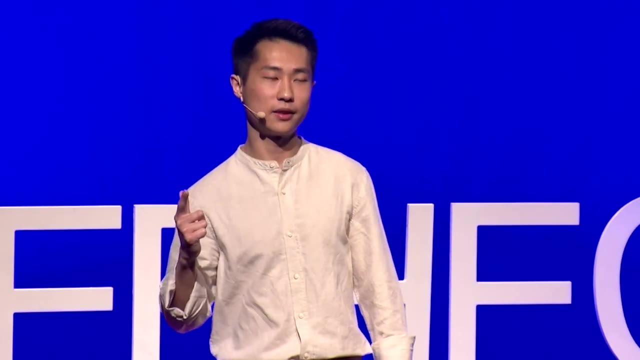 Until now, I shared two ways that I use to better compare to other people. I will call them a smarter way. First, give yourself more time to achieve amazing things. Second, do not just compare yourself at one angle and at their perfect size. 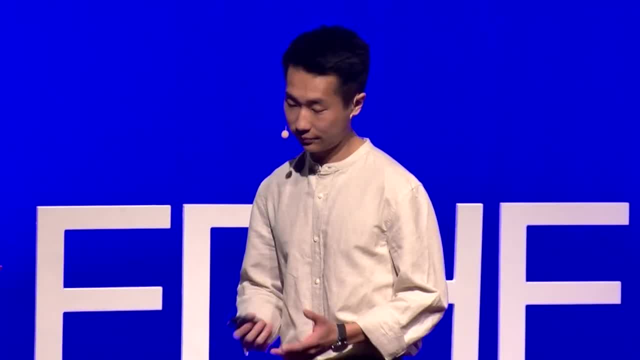 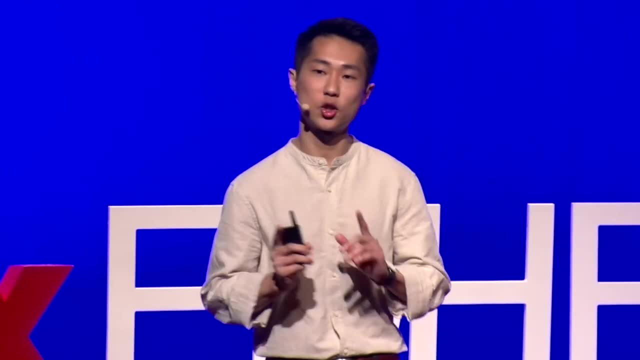 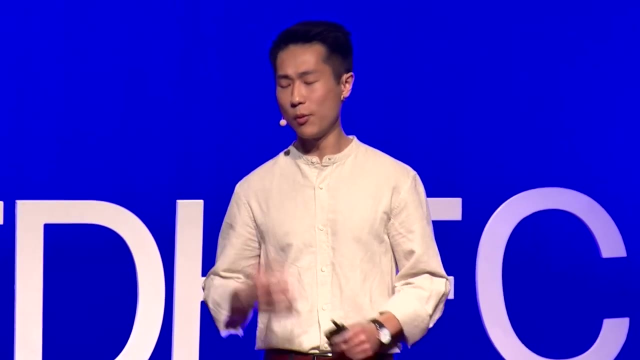 However, it's not enough. The more I grew up, the more I realized that technology- sorry comparison- can be so dangerous because of the fact that it is never ending. I remember when I was young: I wanted to become like my cool classmates. 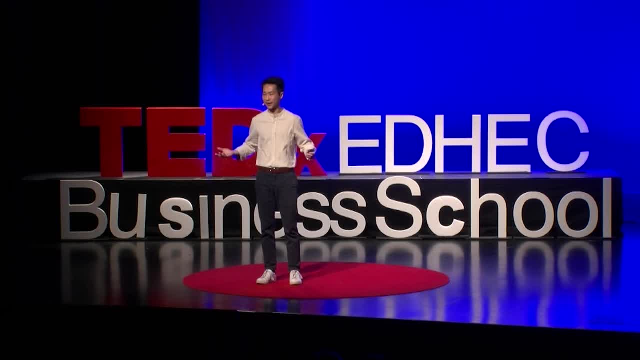 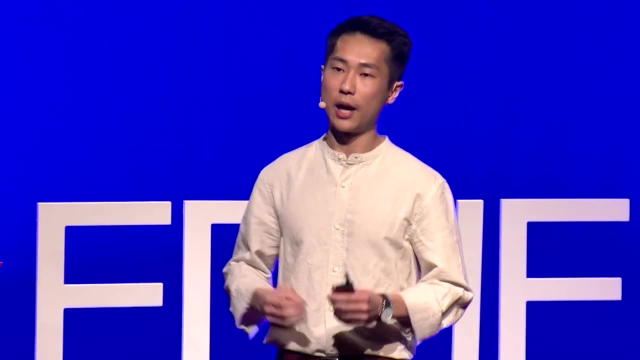 Do you think I became happier when I became like them? No, Because by the moment I became like them, I would have another person that I would compare to and then another person. Comparison is so tiring because our life is completely driven by other people. 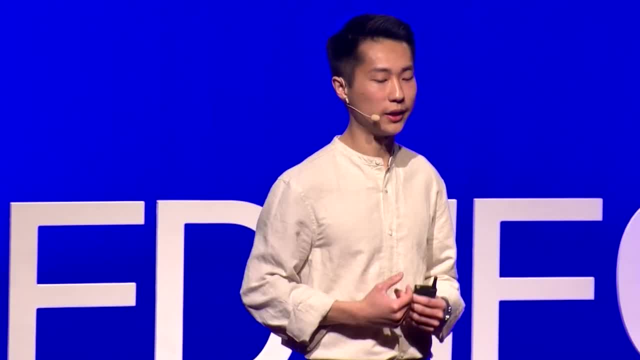 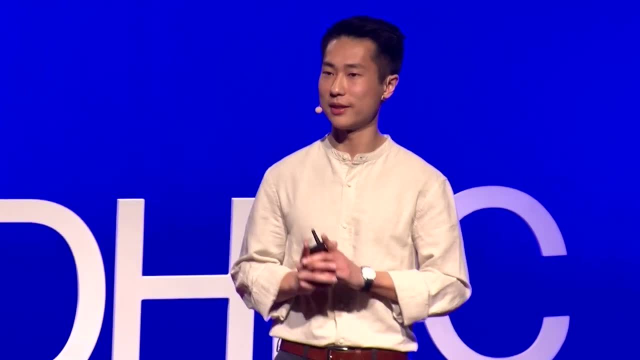 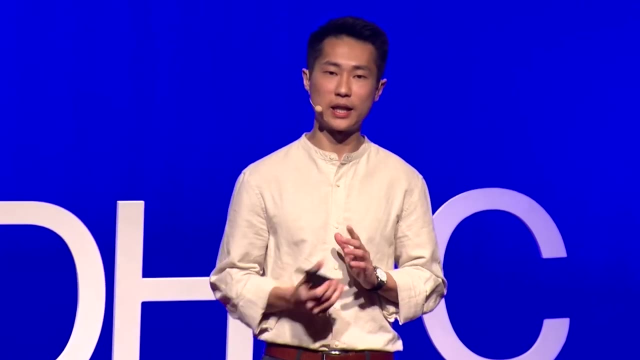 and we seldom really look at our life and appreciate our growth. So here comes to the final, ultimate tip. Instead of spending a lot of time to think how you're worse than other people and compare yourself to other people, try to do one thing. 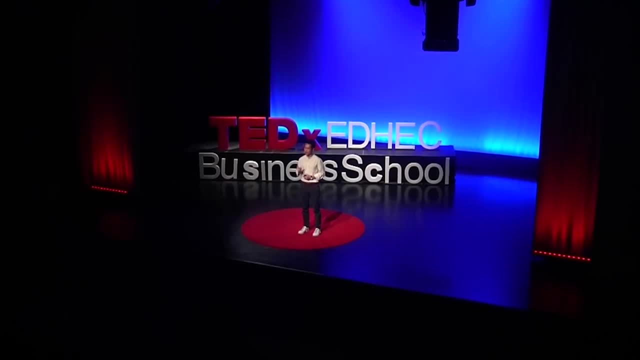 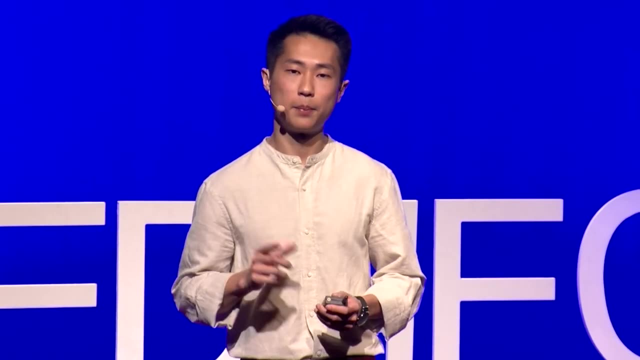 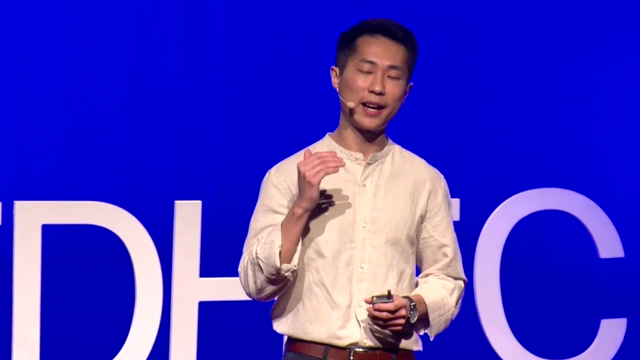 Try to compare yourself to one person, and that is yourself. When I say compare to yourself, what I mean is compare to the same you. but a year ago, a month ago or even a day ago, Are you becoming that kind of person that you aim to become? 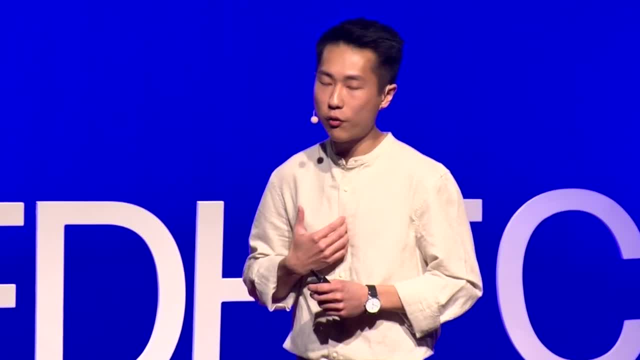 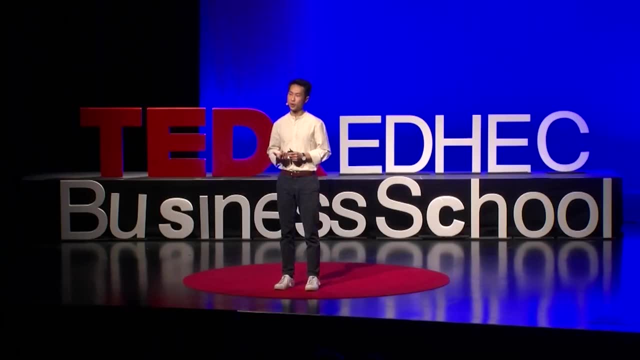 Now, when people ask me how I overcome the comparison in my life, I always tell them the same thing: In my life, what matters the most is not how I am better or worse than other people, but my learnings, my progress. 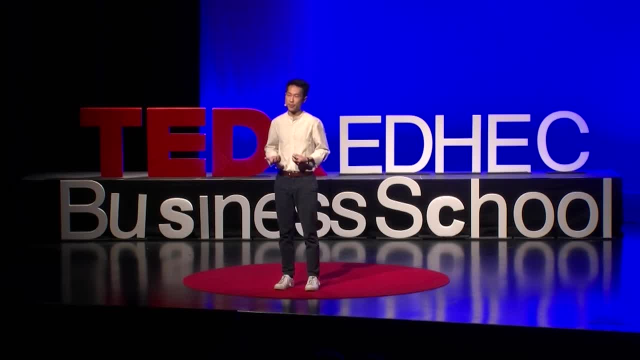 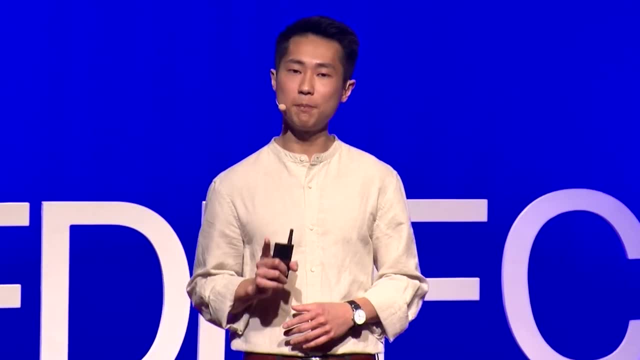 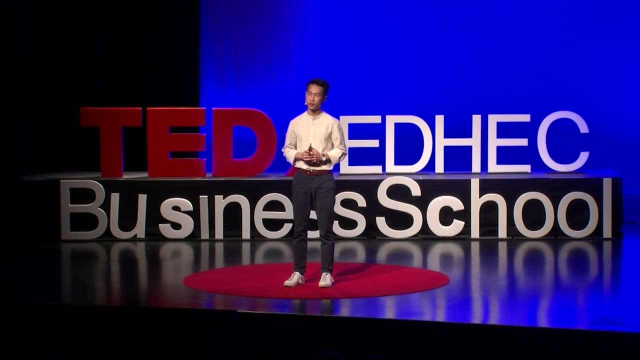 my improvement in my own journey. It has been almost three years now that I came to France and I've never regretted my decision, not because I am better than anyone else, but because I am better than myself. three years ago, So today. 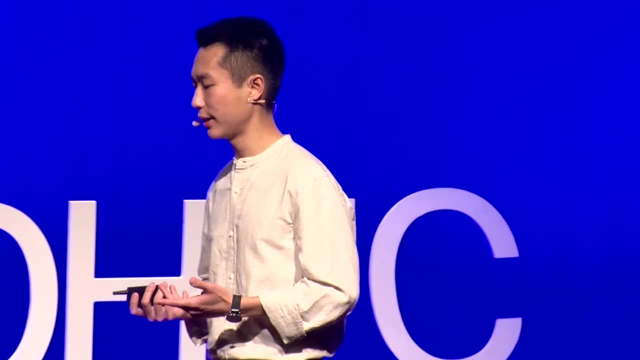 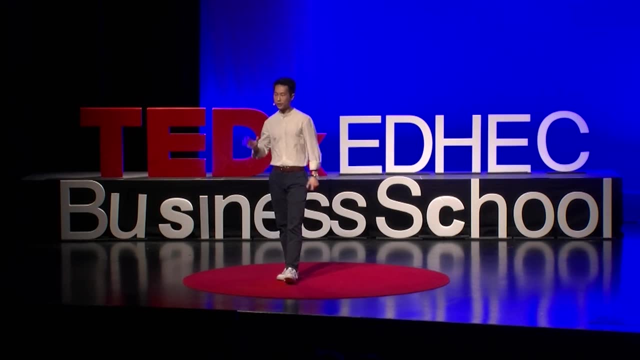 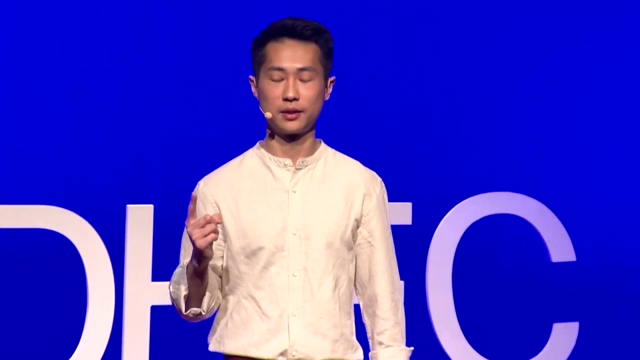 if you tell me that you struggle a little bit in comparison, let's try to do an exercise together, Simple exercise. Now try to use five seconds to think of one thing that you have improved in the past year. It can be I became better at coding. 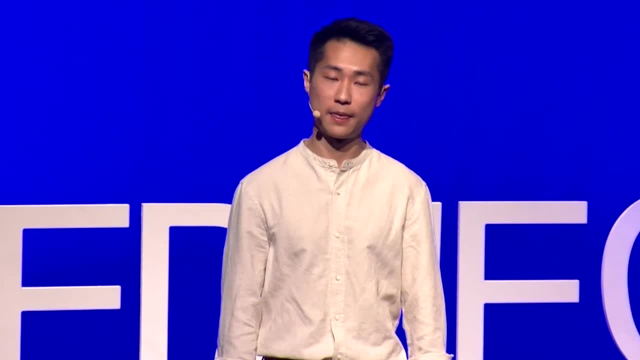 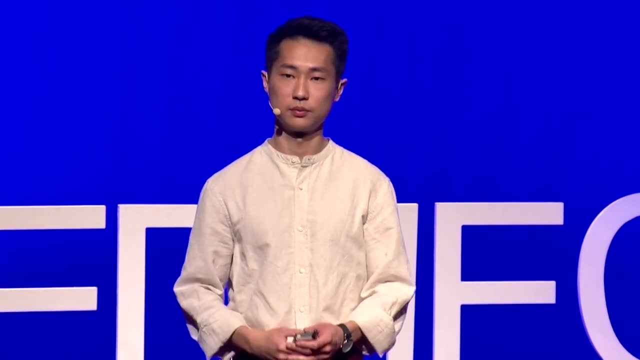 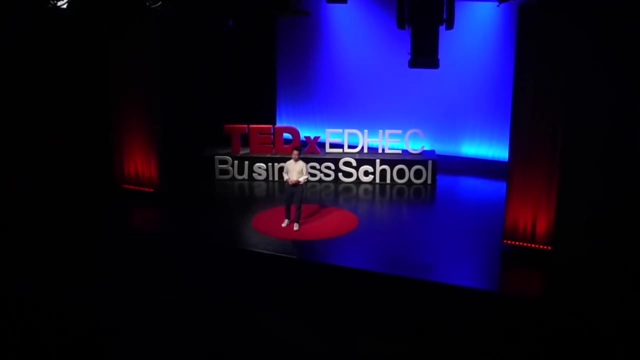 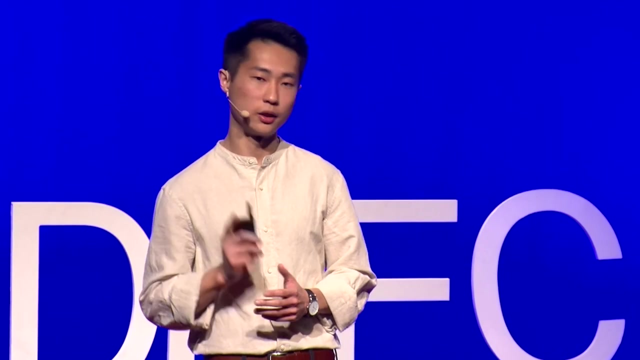 or I read more books last year. What about you? Five seconds, one thing that you have improved. I believe that in these five seconds, many of you can think of something that you have improved in the past year. Try to focus more on that. 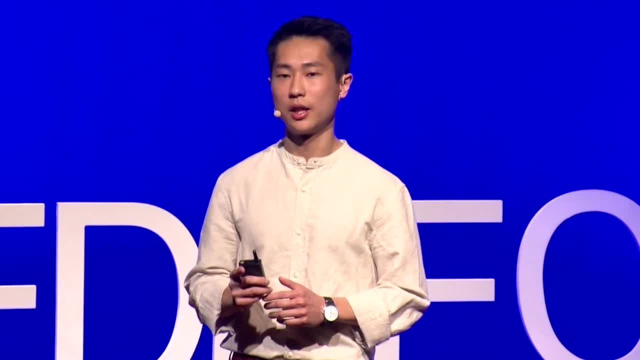 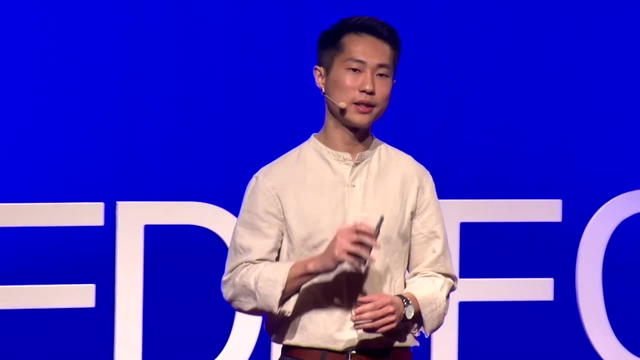 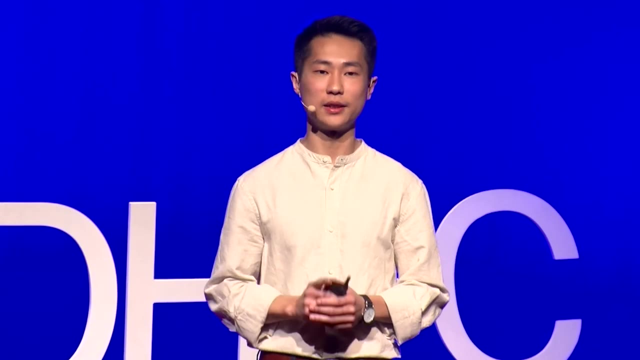 because that's something that matters the most in your life. Try to appreciate more your growth. At the end of the day, you are not living in anyone else's life, but your own life. After this speech, I encourage you all to do one thing.